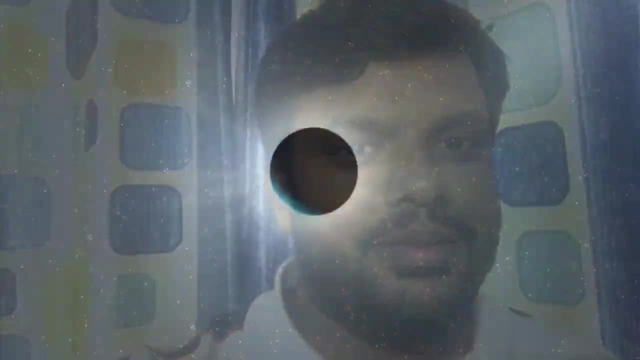 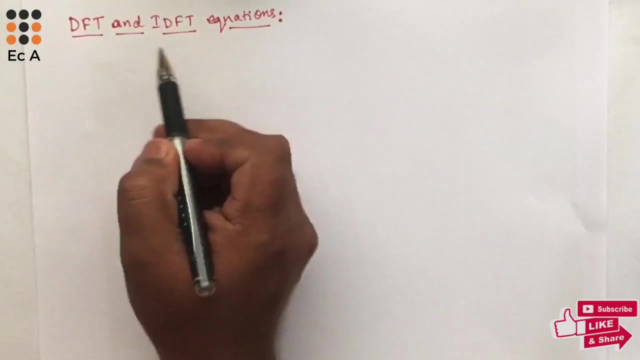 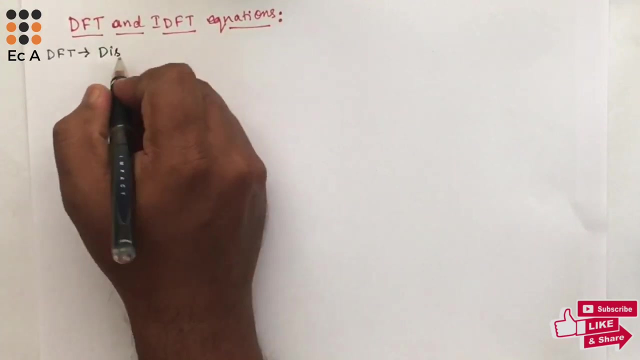 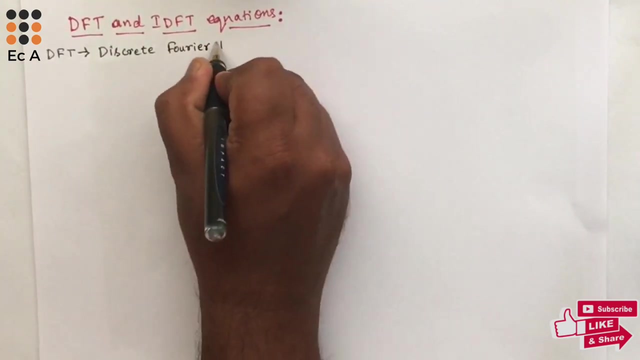 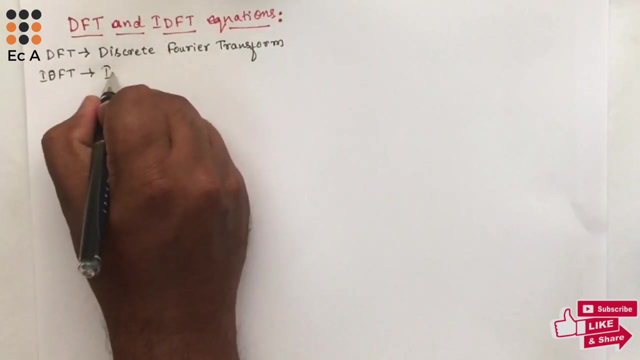 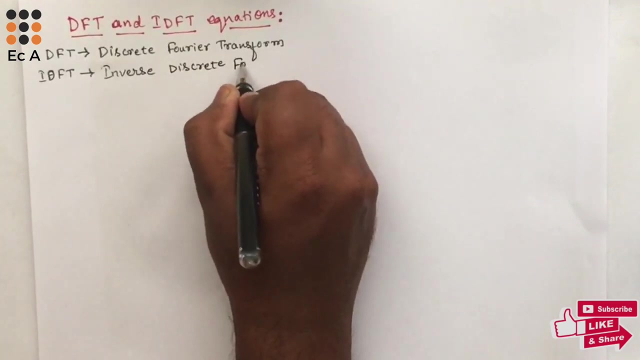 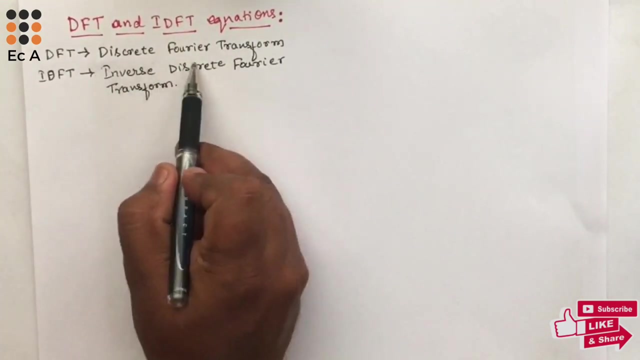 Hello friends, welcome to EC Academy. In this lecture let us understand DFT and IDFT equations. DFT is nothing but Discrete Fourier Transform and IDFT is nothing but Inverse Discrete Fourier Transform. So DFT is Discrete Fourier Transform and IDFT is Inverse Discrete Fourier Transform. 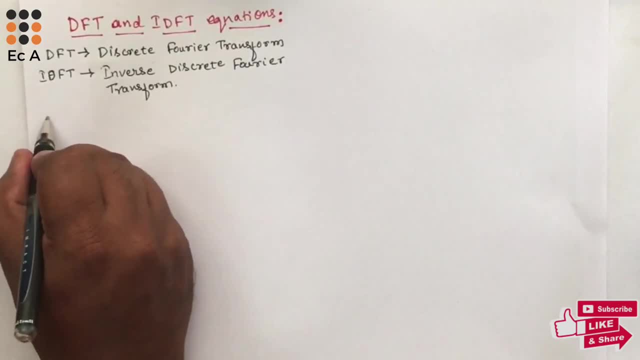 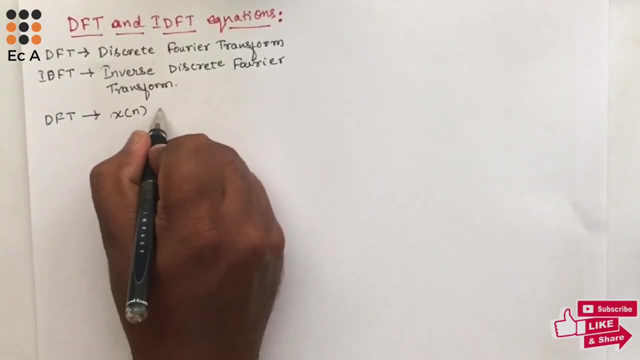 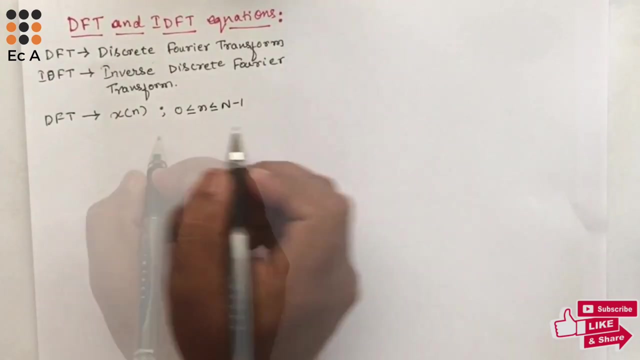 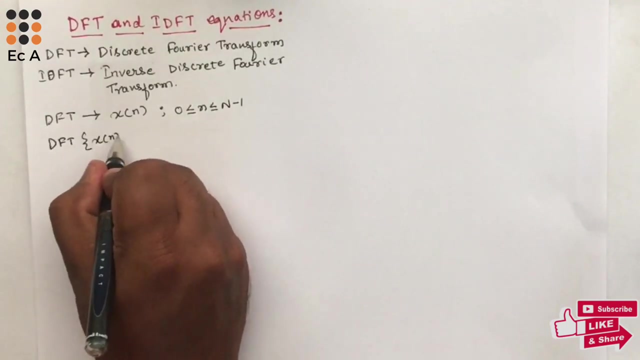 First let us see the equation for DFT: DFT of a finite length, sequence x of n, where the value of n ranging between 0 and n minus 1 can be given as DFT of x of n, which is equal to x of k. 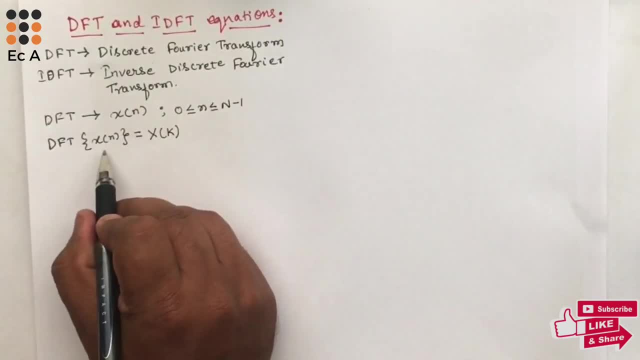 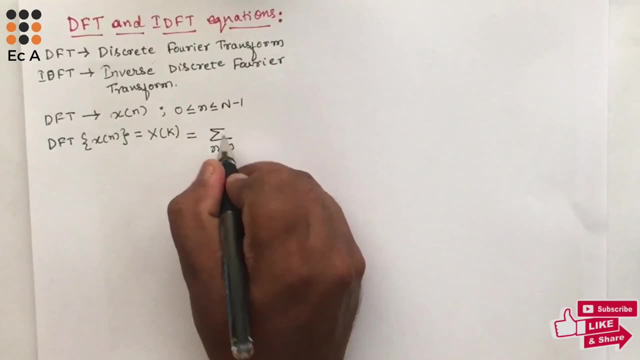 So x of k is DFT of x of n. that can be given as: summation of n is equal to 0 to n minus 1, x of n, e to the power of minus j, 2 pi by n into k, n. here the value of k is ranging between 0 to n-1.. 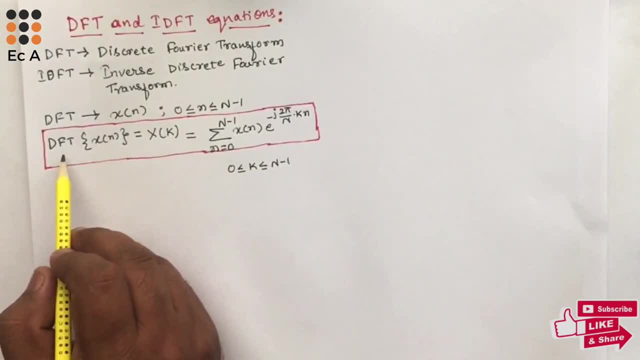 This is the equation for DFT, so this equation is derived from equation number 5. if you can remember the lecture number 2, we had equation number 5, where we have written x two pi by n into k, x 2 pi by n into k. 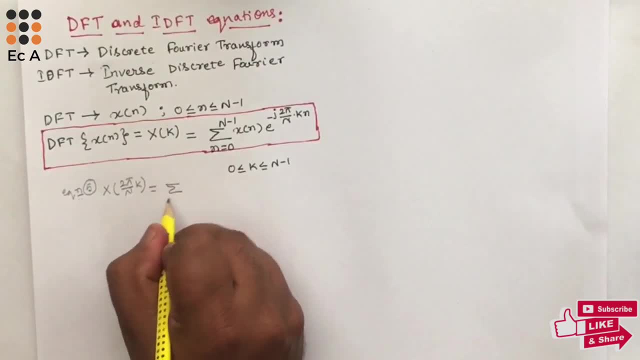 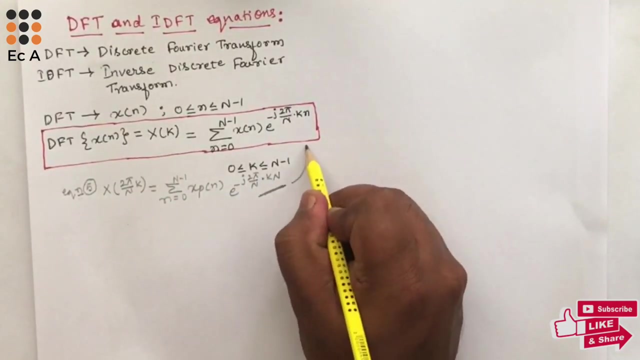 x 2 pi by n into k equal to summation of n is equal to 0 to n. minus 1 x p of n e to the power of minus j. 2 pi by n into k n. So using this equation we have written the equation for DFT. So here: x of 2 pi by n. 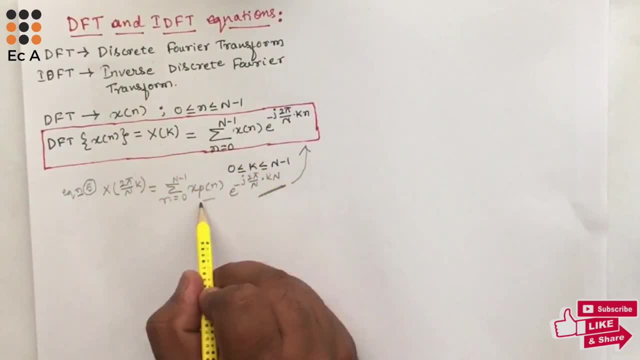 into k. we have written it as x of k and x p of n is written as x of n. I will rewrite the above equation and write it as: DFT of x of n is equal to x of k. that can be written as summation of: 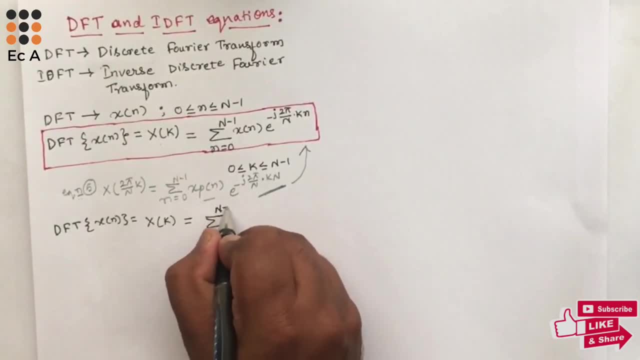 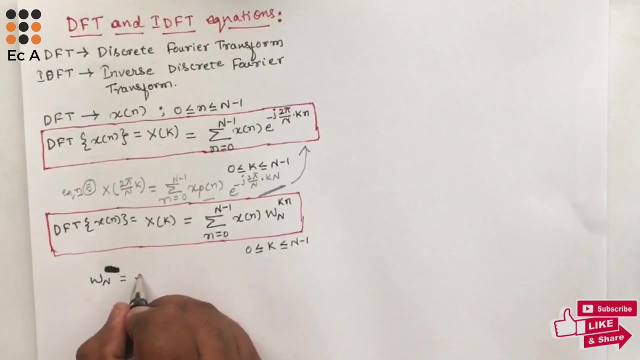 n is equal to 0 to n minus 1 x of n into omega n, to the power of k n. Here again, the value of k is ranging between 0 to n minus 1.. In this equation, omega n is equal to e, to the power of minus j, 2 pi by n. So 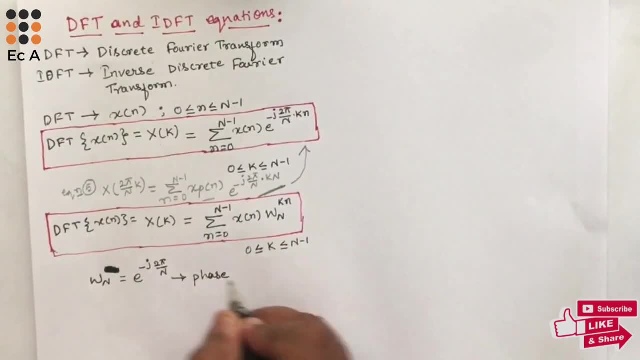 this is nothing but phase factor, or it is also known as twiddle factor. In both the equations x of k is sequence in frequency domain and this sequence also known as luminance, So by 필lyalon equation i would take in Paulin. 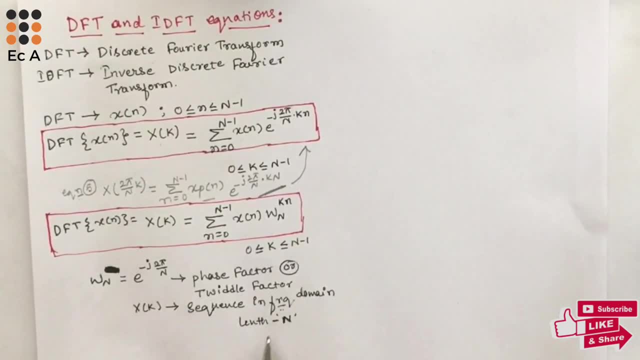 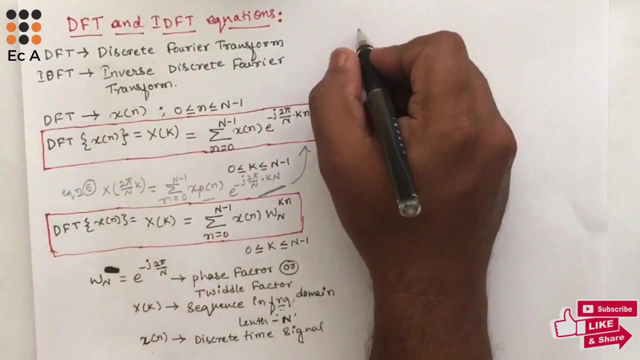 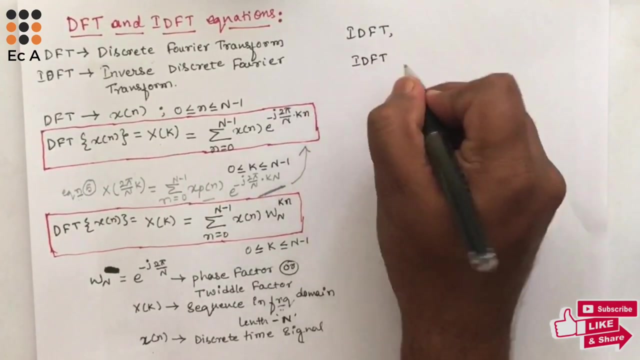 the Tyson Meghanγοne equation that cos j 3 by n is equal to 0 into k. Now capital X of k is equal to. if we take IDFT of capital X of k, we will get X of n. that can be: 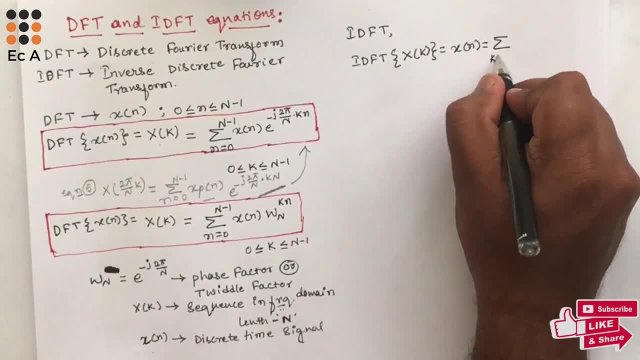 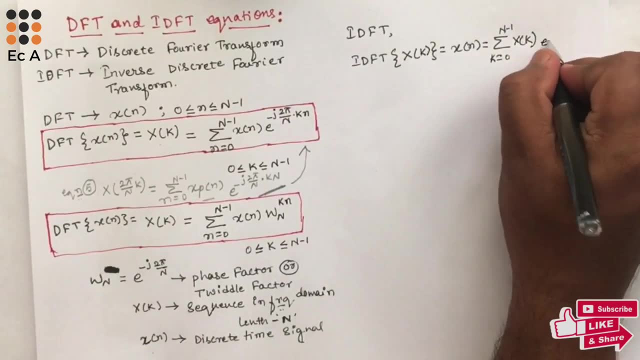 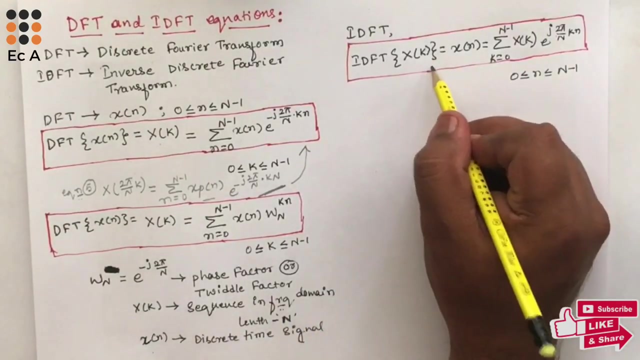 written as: summation of k is equal to 0 to n minus 1, X of k, e to the power of j, 2 pi by n, k, n, where n varies between 0 to n minus 1.. If you can remember, this equation is written from: 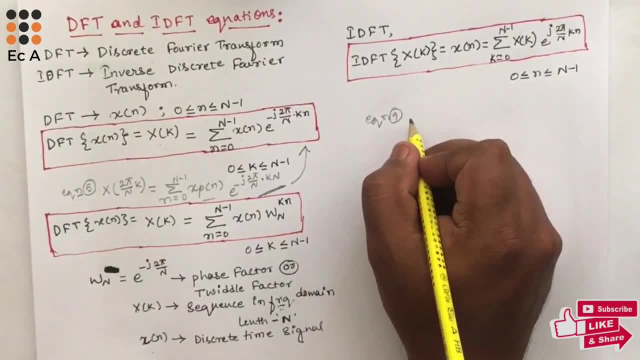 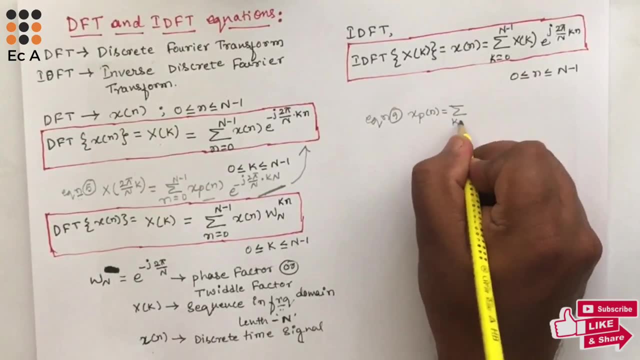 equation number 9 from our previous topic in lecture number 2, where we have written X p of n is equal to summation of k is equal to 0 to n minus 1. X of 2 pi by n. x of 2 pi by n.